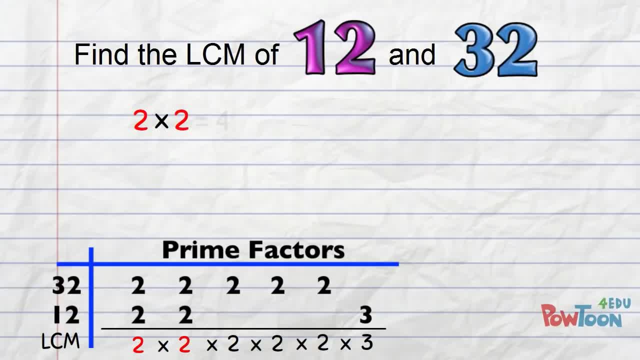 Work it out: 2 times 2 is 4 times 2 is 8, times 2 is 16 times 2 is 32. 32 times 3. 3 times 2 is 6. 3 times 3 is 9. 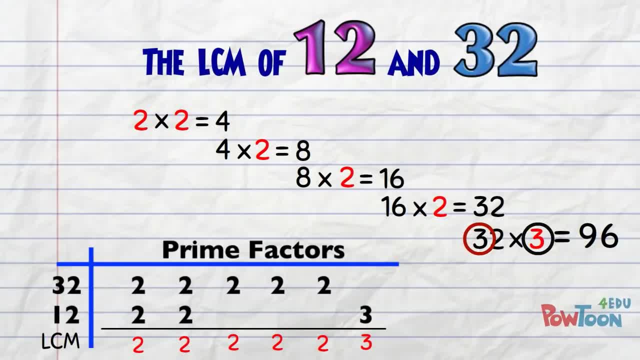 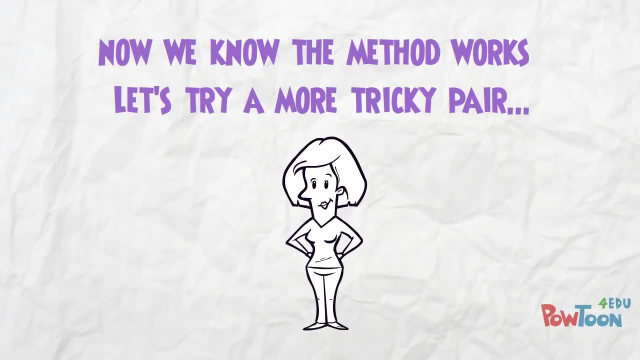 So the LCM of 12 and 32 is 96. And we know this is right because we already found the LCM using the multiple listing method. Now we know the method works, let's try a slightly more tricky pair: 28 and 35. 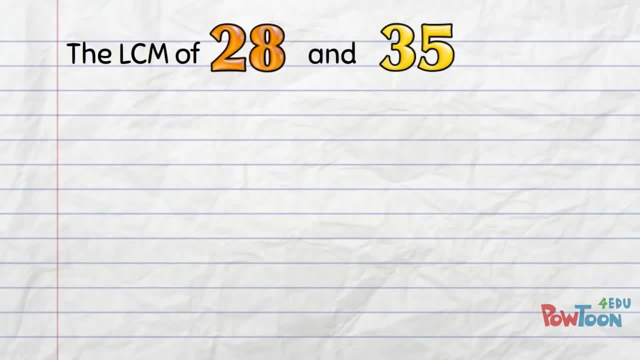 First find the prime factors of each number. 28 is from 4 times 7, 4 is from 2 times 2, Circle the primes 35 is from 5 times 7, Both prime. Next we do the prime factors table: Match factors vertically. 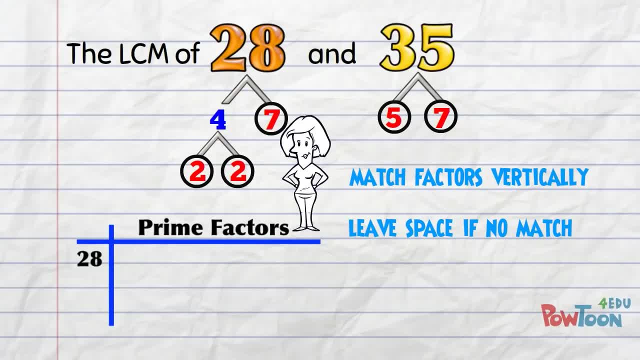 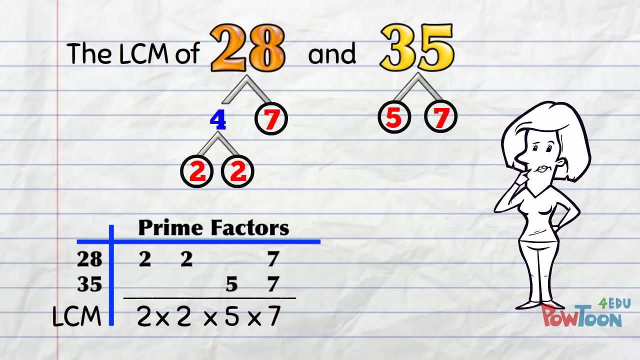 Leave a space if there's no match. 28 is 2 times 2 times 7, 35 is 5 times 7. Now we get the prime factors of the LCM: 2 times 2 times 5 times 7. Finally, work out the value of the LCM. 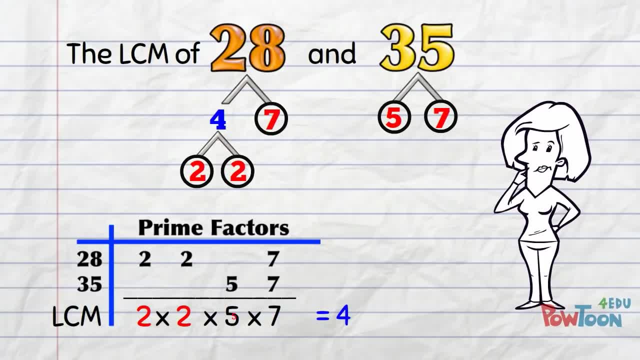 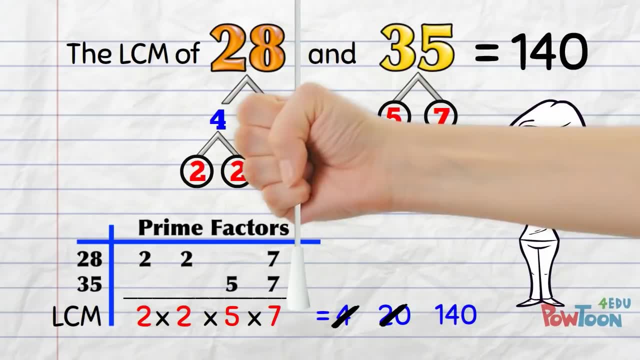 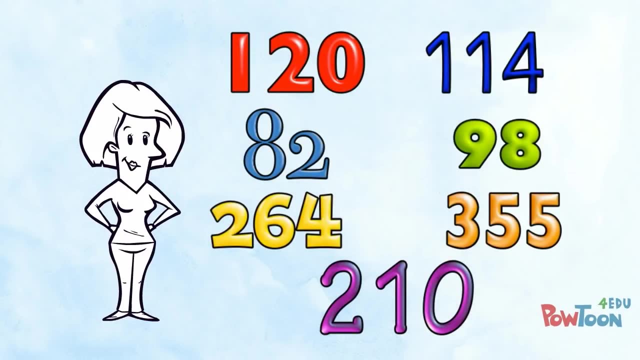 2 times 2 is 4 times 5 is 20 times 7 is 140. You can see when you are given even bigger numbers. using the prime factorization method is going to be very helpful. Now here's a challenge for you. 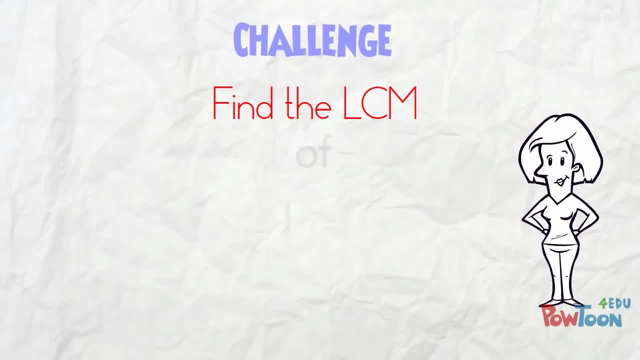 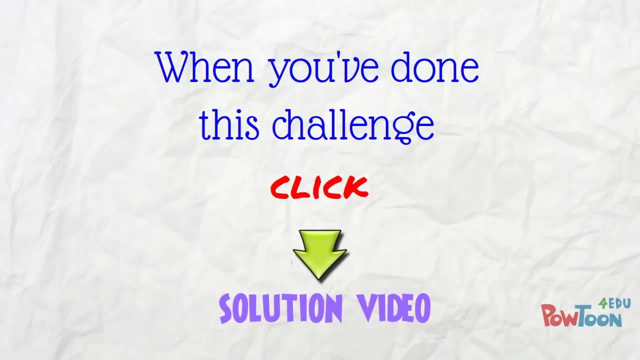 Using the method I just showed you, find the LCM of 15,, 32 and 66. You can do it. When you've done this for yourself, click the link here to check my solution video and see if we got the same answer. 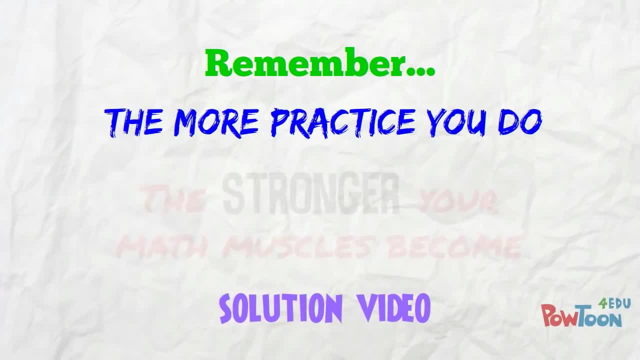 Remember: the more practice you do, the stronger your math muscles become.